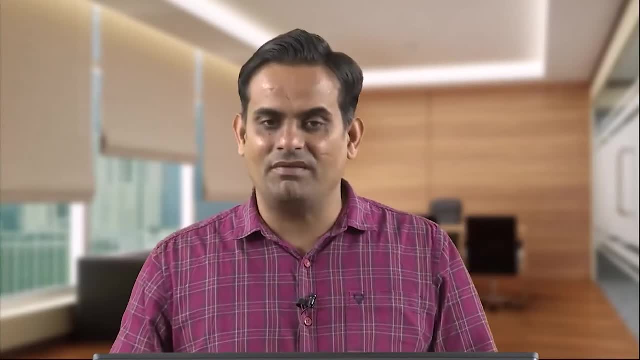 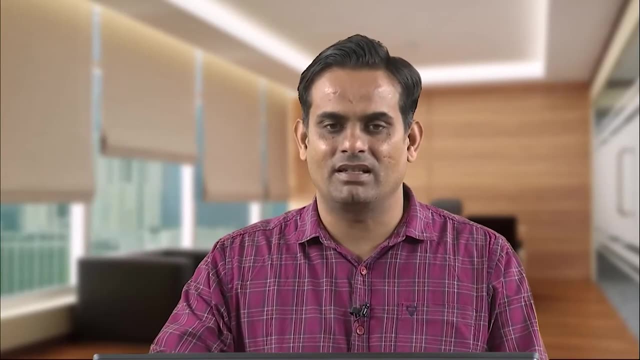 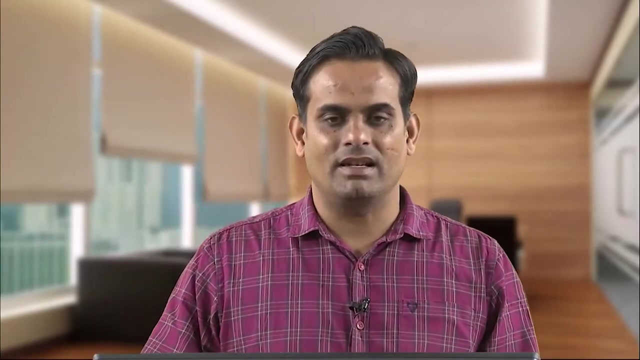 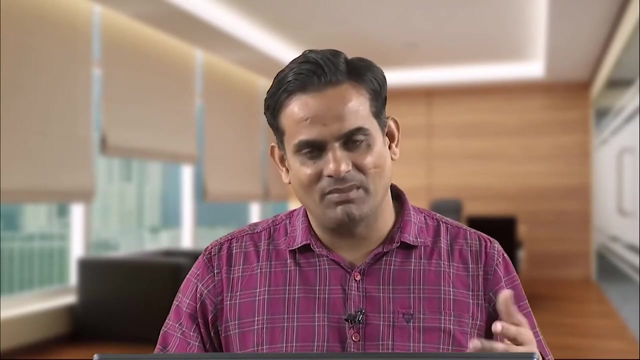 related to singular value decomposition. However, we are having a very important application of singular value decomposition, which we will discuss in this lecture, and that is called low rank approximation. So first we will start this lecture with the definition, So definition of rank. However, we have taken rank in previous lectures and by this 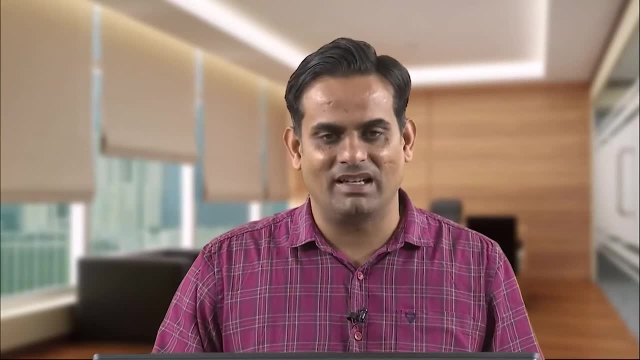 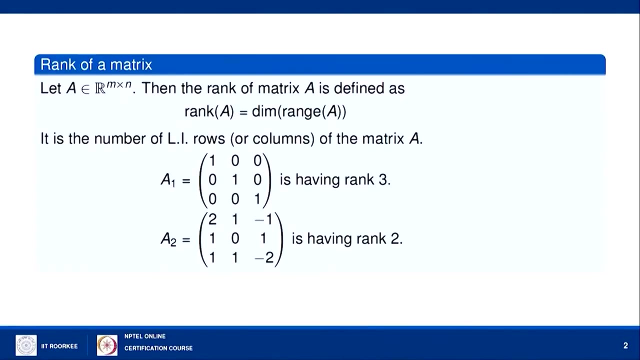 time. you know very well what we mean by rank of a matrix. However, again let me define it. So let A be a m by n- real matrix, then the rank of matrix is defined as the dimension of range space of A and the similarly dimension of null space is called the nullity. But here 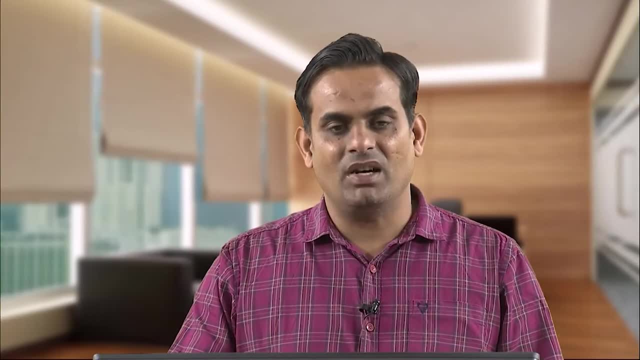 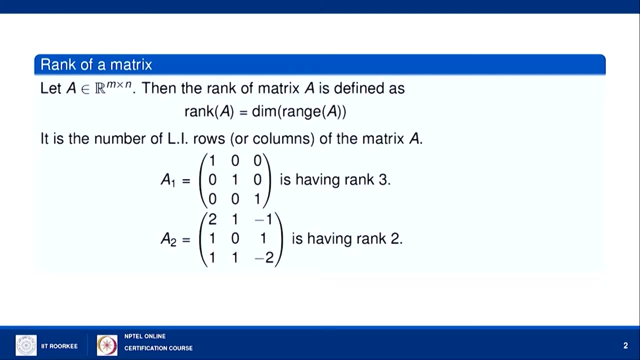 we are focusing on rank. It is the number of linearly independent rows or columns of the matrix A. So, for example, if you take this matrix, so it is an identity matrix and it is having 3 linearly independent row or 3 linearly independent columns. So rank of 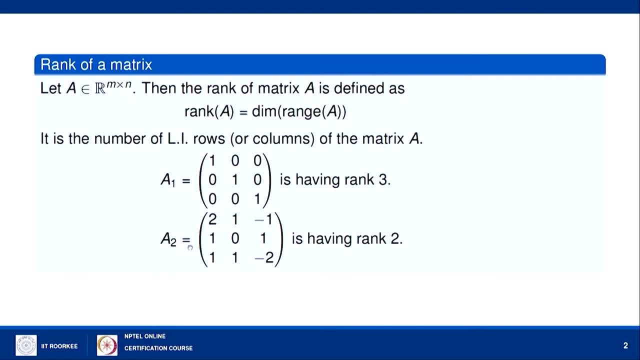 A1 is 3.. Similarly, if you see this, A2, so here, if you see this in this form, we cannot say about the linearly independent or linearly dependent. However, if you carefully check it, if I subtract second row from the first one, what I will get? 2 minus 1, 1, 1 minus 0, 1. 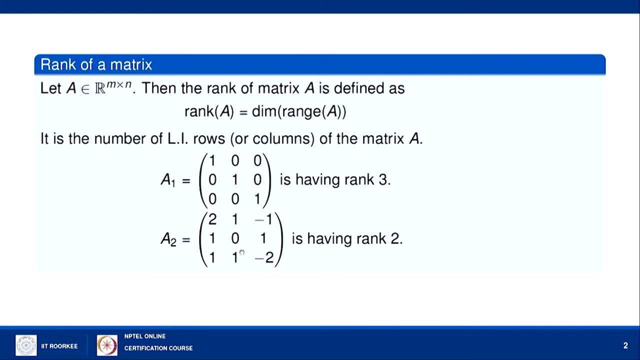 minus 1 minus 1 equals to minus 2.. So third row is nothing, just it is depending on the first two rows. that is, third row is the R 3, that is, the row 3 equals to row 1 minus row 2.. So all three rows are not linearly independent, one row depending on the linear. 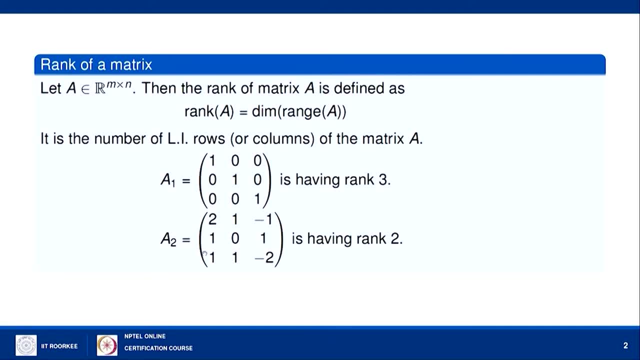 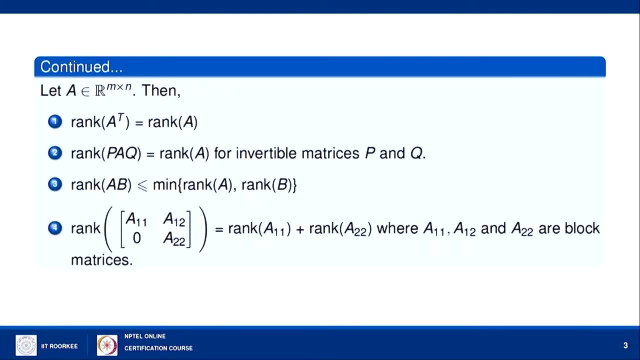 combination of other two rows. Hence the rank of this matrix is 2.. So this is all about the rank. then we are having some of the important property about rank. one of the properties: rank of the parity field of A equals to rank of A transpose, and that is why I am saying row rank equals to column. 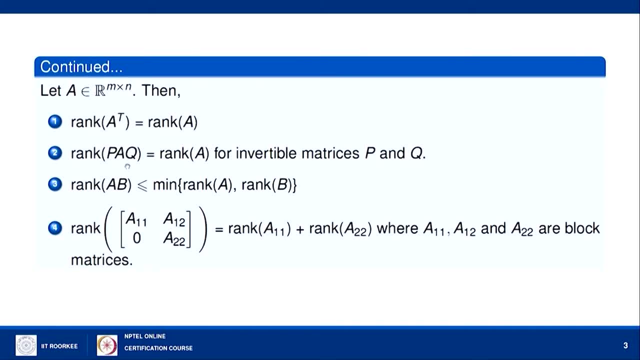 rank. Rank of a matrix- P, A, Q- equals to rank of A for any invertible matrices, P and Q. So if P is invertible, Q is invertible, then rank of the product of P, A, Q equals to rank of A. Then we are having so, like in the case of singular value decomposition we have seen. 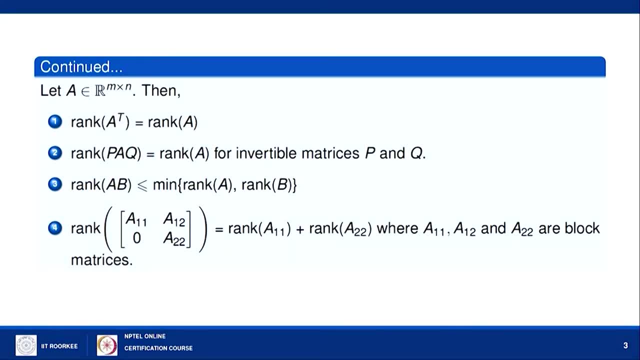 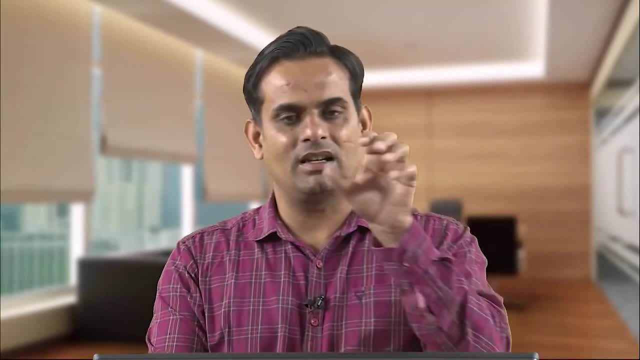 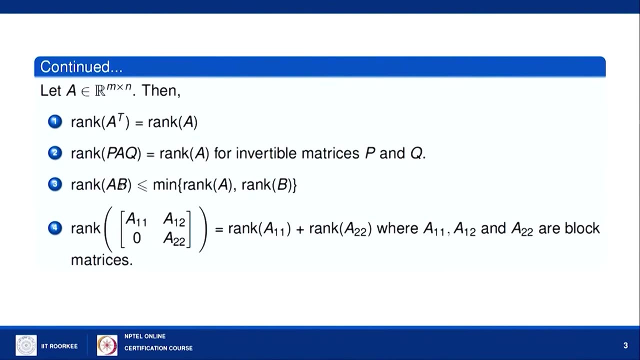 that rank of A equals to rank of sigma. That is why we are saying the rank of A equals to the number of nonzero singular values, that is, the number of nonzero rows or nonzero columns, Because they are u and v transpose, are orthogonal matrices and they are invertible. 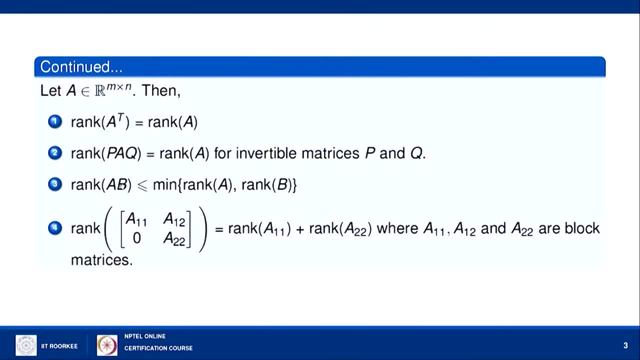 My third property is rank of the product of two matrices, A and B. That is, rank of A B will be always less than equals to minimum of rank A comma rank B. Fourth one is: if you are having this kind of block matrix where A 1- 1 is a block matrix, A 1- 2 is a block. 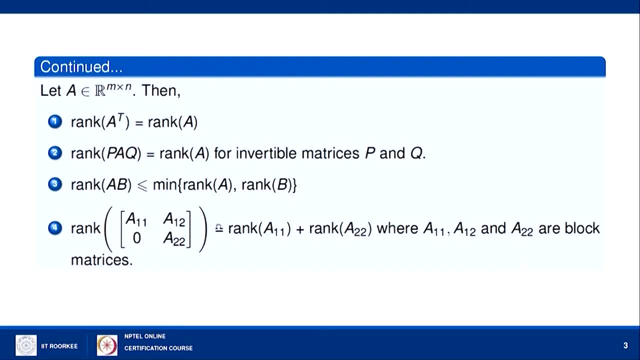 matrix A 2- 2. this equals to greater than equals to. sorry, it will be greater than equals to In the case when A 1- 1 and A 2- 2 are zero matrices. So rank right hand side will be zero. However, left hand side will depend on the rank of A 1- 2.. So this make this correction. 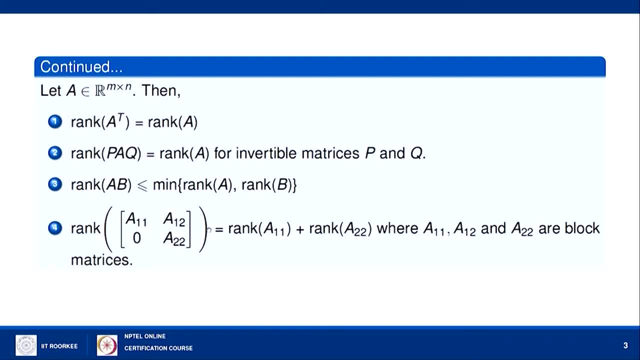 it is greater than equals to where all these A 1- 1, A 1- 2 and A 2- 2 are block matrices. So these are some of the important properties about rank which we can remember easily and we will use these very frequently. 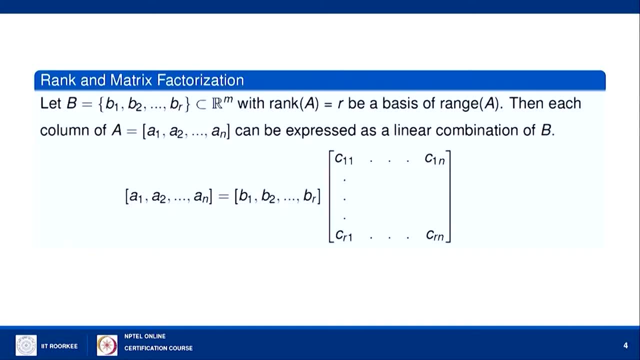 Again, we have used these properties earlier, also now matrix spectrization and its relation with the rank. So let B having vectors B 1,, B 2, B r, all are m dimensional vector, So B be a set of vectors and we are having rank of A equals to r, where A is a m by n. 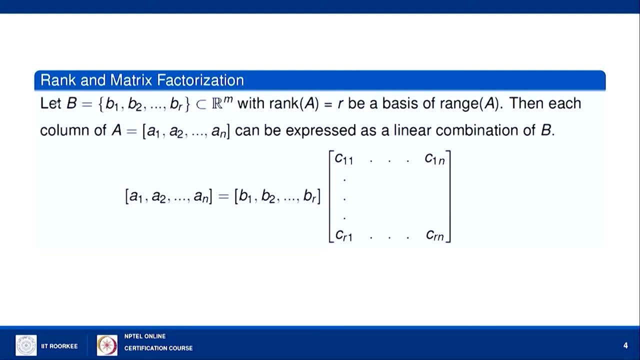 matrix be a basis of range space of A. So matrix A is m by n matrix. So it is a linear transformation from R n to R m. So obviously range space will be a subspace of R m and that is why. 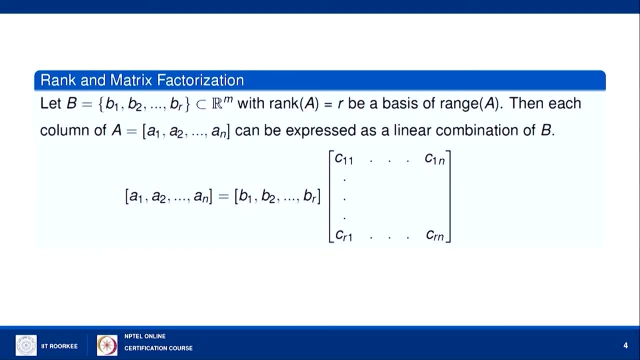 we are taking these b 1, b 2, b r, as the m dimensional vectors are linearly independent vectors. Now then, each of the column of this matrix A can be expressed as a linear combination of B, How a 1, a 2, a n equals to b 1, b 2, b r, and then columns of C 1, C. so So now, 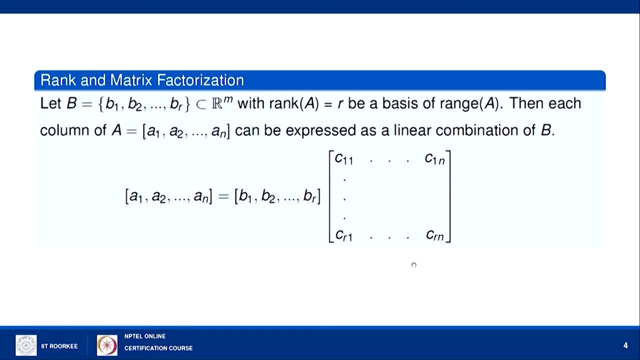 this matrix C is called the basis matrix, So these columns are the basis and these are giving the coordinates. So if you want to make first column, first column, First column will become b 1, C 1, 1 plus b 2, C 1, 2 plus plus up to b, r, C, r 1 and. 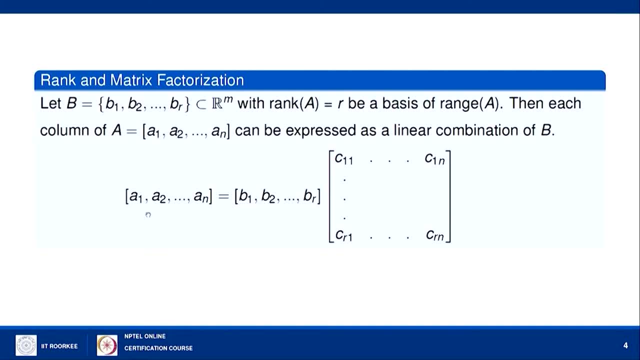 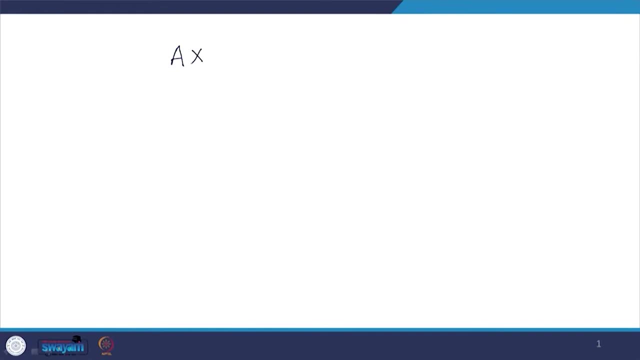 that will be our a 1.. So in that way we will be having all the columns of A as the linear combination of B, And that you can see very easily because we are having, if you consider the linear system, A x equals to B or A: x equals to b. 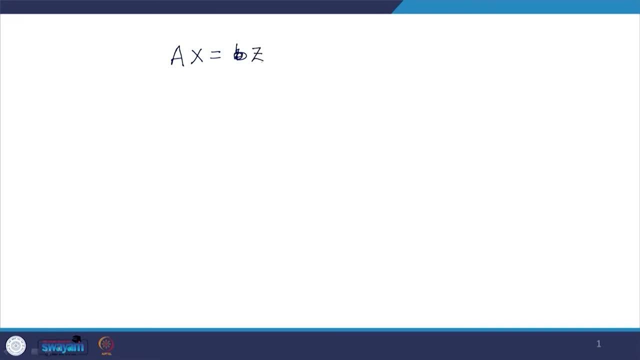 So suppose aз equals to- let us not right A- x equals to z, So z is right hand side vector. this system will be having a solution when rank of A equals to rank of augmented matrix A- z And when it will be having unique solution when this is equals to the number. 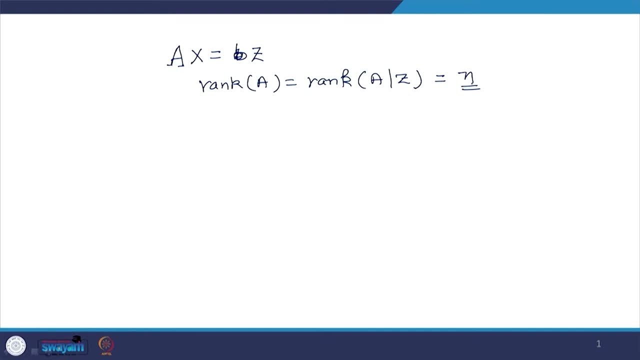 of unknowns, that is x, otherwise it will be having infinite number of solution. So if So, if rank of A is equals to R, which is less than N, so let us say it is less than equals to N in that way. So what will happen? If you can write the columns of A and then you 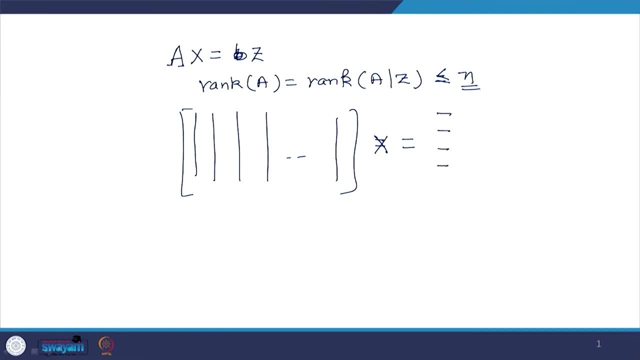 are having X and here you are having this Z. So if you can write this Z as the linear components of columns of matrix A, then the system will be having a solution. and what will be that solution? Solution will be the coordinates of that linear combination. 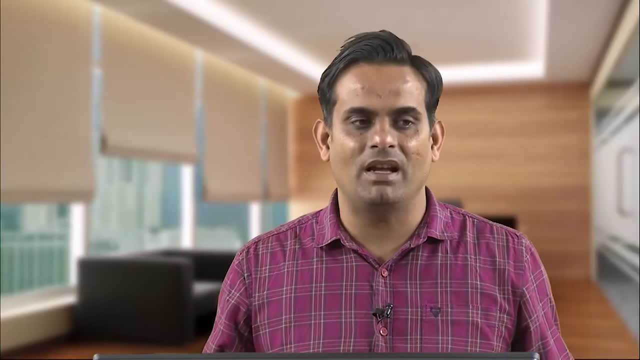 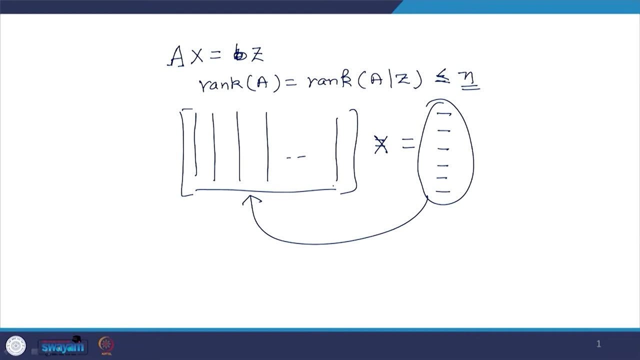 So if you can write it uniquely, then you will be having the unique solution, and when you can write uniquely, when it is a full rank matrix- If you cannot write it uniquely means you can write in different way- then you will be having more than one solution. 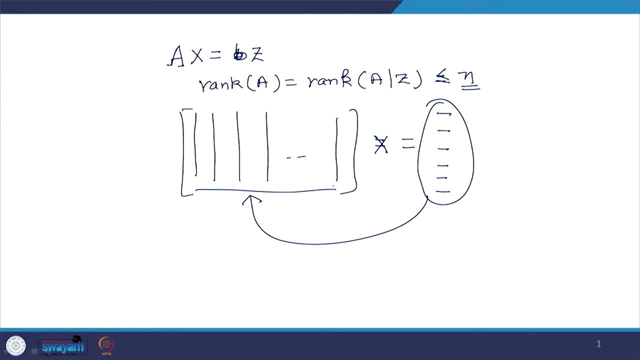 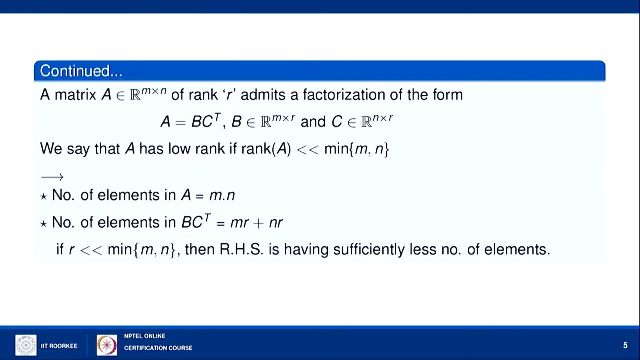 And that is the infinite number of solutions. and when you will be having that? when this is not a full rank matrix. So in that way we can visualize this concept. So we are saying that if A is a M by N matrix, rank of A is equals to R, then we can have 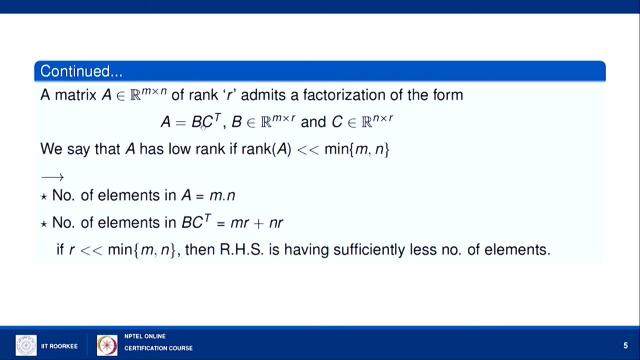 a factorization of A, as A is equals to B. C transpose means we are writing the columns of A as the linear combination of product of the basis of the range space of A, and then a matrix C, And here B is M, by R matrix, because you are having R vectors, each one of M dimension. 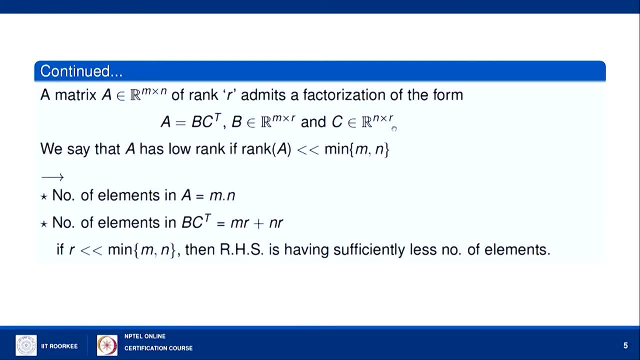 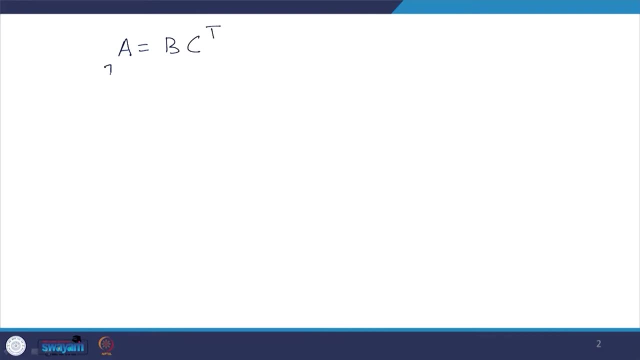 and C is a, N by R matrix, then this particular product will be well defined. So what I am saying? I am saying A equals to B, C transpose. where is A is M by N, B is M by R and C transpose is R by N. So now what we are saying. if you see carefully, number 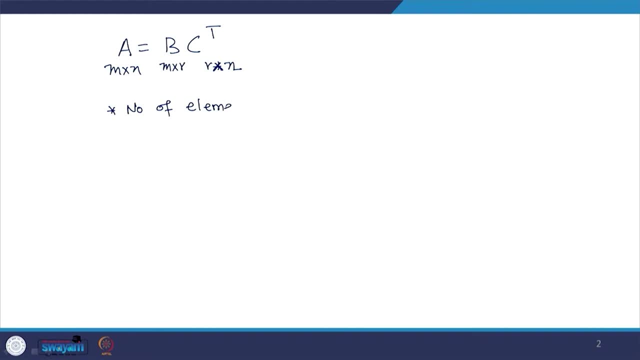 of elements in A equals to m times n number of elements in B into C. transpose. So in B you will be having m into r elements. plus in C transpose you will be having n into r elements. Now consider a situation where A is a 50 by 100 matrix with rank of A equals to. let us 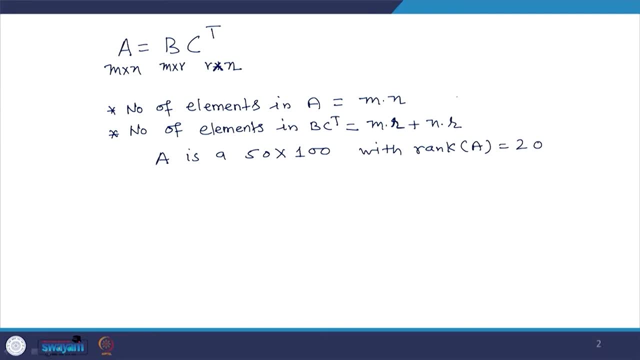 say 20.. So how many elements you have to store here for writing this matrix means you have to save. how many elements you have to store 50 into 100, that is 5000 elements. However, in this case, how many elements you require to save 50 into 20, that is 1000 plus 100 into. 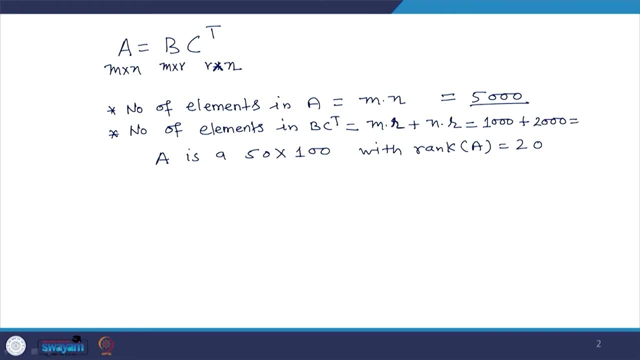 20, that is 1000.. So only 3000.. So now, if you see this, this is the motivation of low rank approximation. So in original case you have to save 5000 elements, but in this case you have to save. 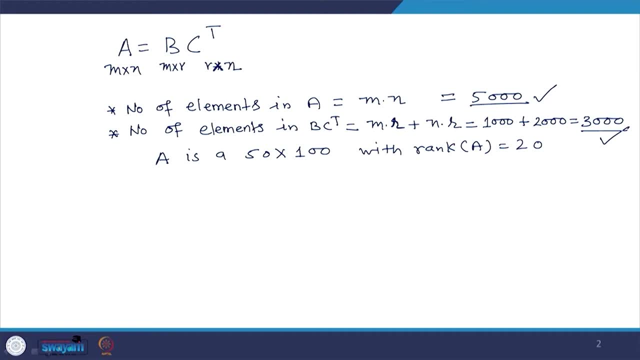 only 3000 elements and you are saving the same thing, that is, the matrix A. So in that way you can save the memory elements. Ok, Thank you. Thank you as well as the computational cost, Because if you want to operate something on this matrix, 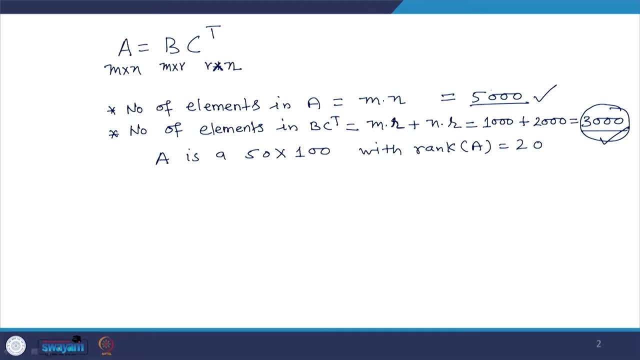 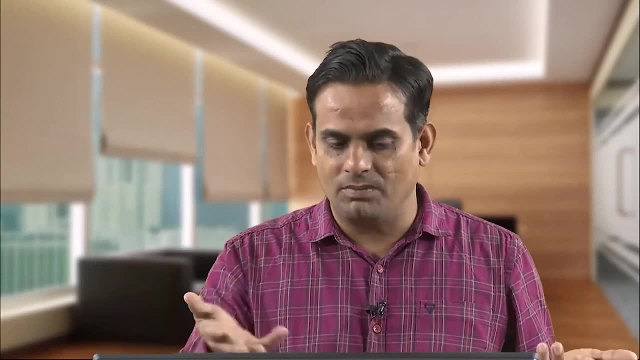 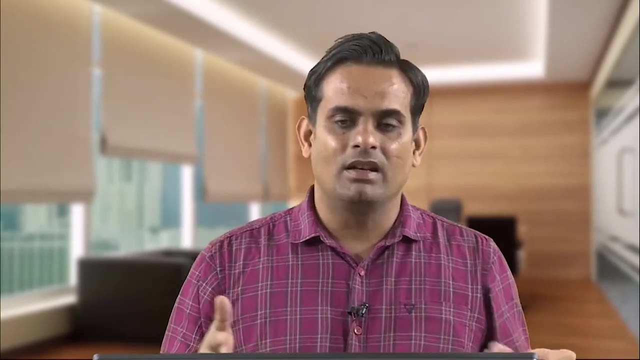 A. you want to process this matrix, you have to process all the 5000 elements. means if it is an image, digital image, you will be having 5000 pixels in A. But in case of, if you are writing it in this way, B into C transpose, then you have to play with only 3000 pixels. 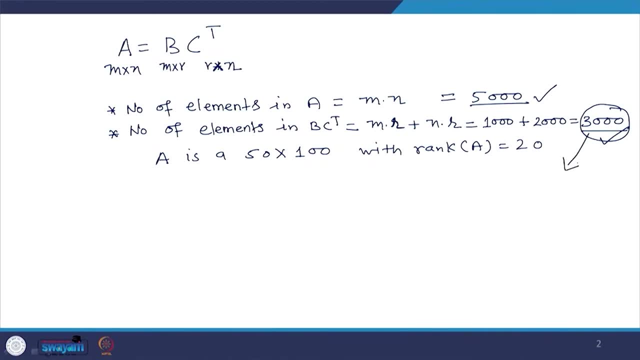 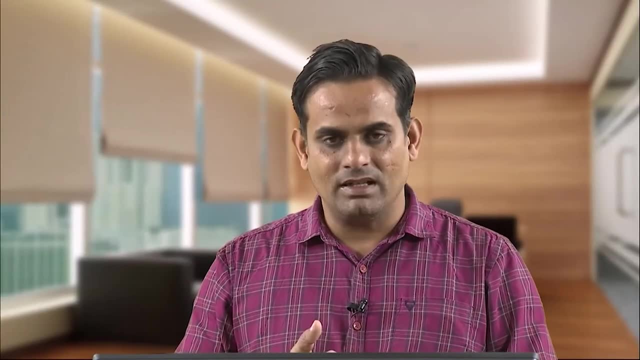 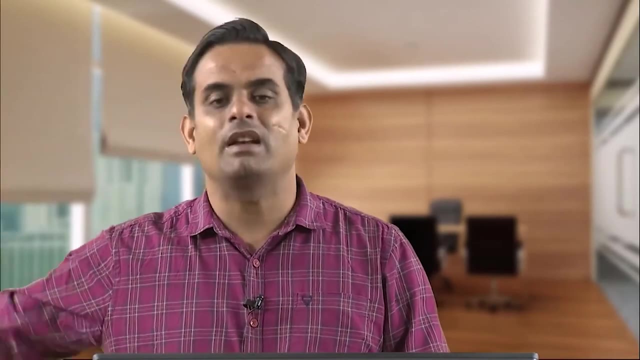 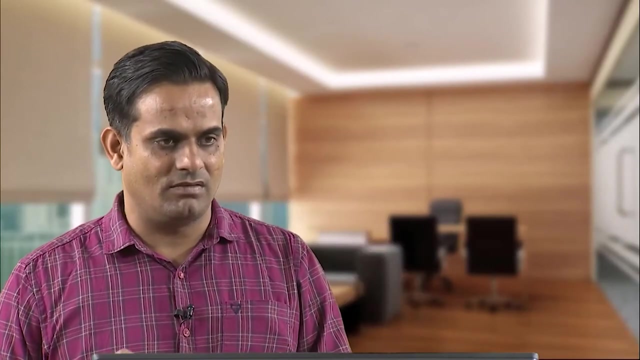 So this is a motivation for low rank approximation. Given a matrix or a tensor, you find out another matrix or tensor which is having the lower rank to the original one and the same time it is quite close to the original one. So, based on this motivation, let us define the 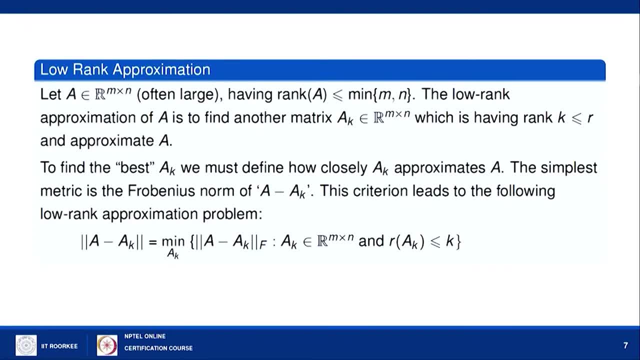 low rank. So let A be a M by N matrix and it is large, because if matrices are very large, then only we talk about low rank approximation, Having rank of A which is less than equals to minimum of M or N. The low rank approximation of A is to find another matrix, say K, of the same. 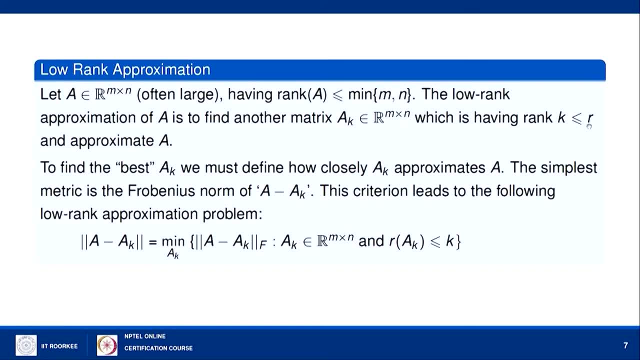 size, which is having rank K less than equals to R. So size will be same. but again, if rank is lower, that is, the rank is K, which is the rank of the original matrix A. Then I can write save this matrix easily with the lower number. 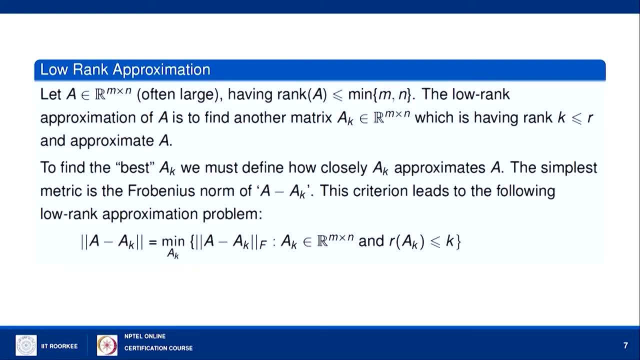 of entries by using the matrix factorization which we have seen in the earlier slide, So which is having rank K, which is less than equals to R, and approximate A. Now to find the best A K, we must define how closely A K approximate A. 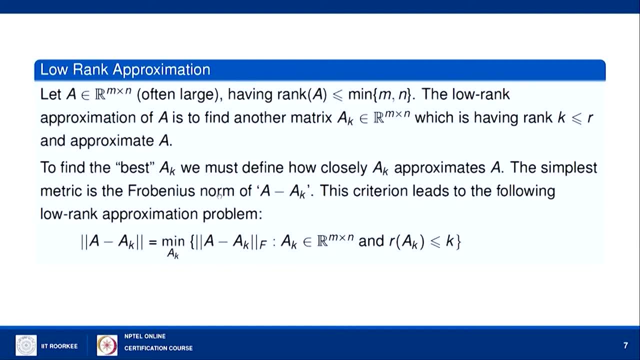 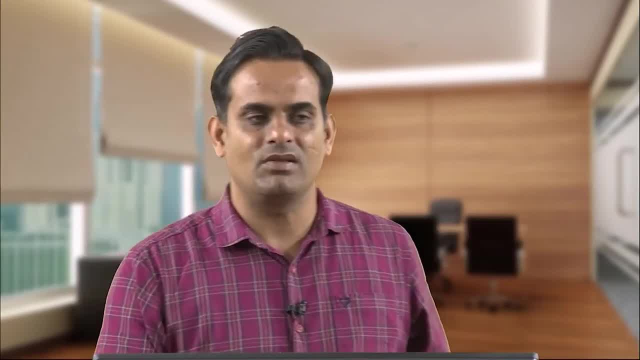 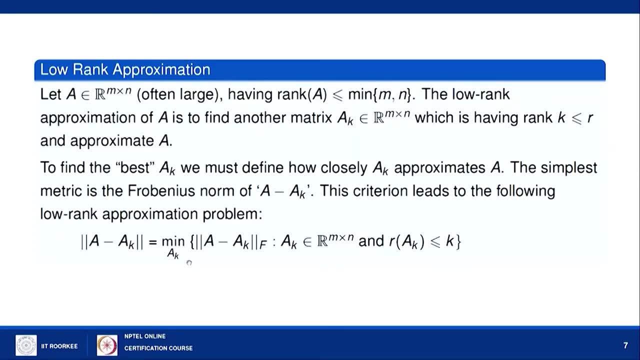 The simplest matrix is the Frobenius norm of the difference of these two matrices, that is, your original matrix and the matrix which you are approximating. This criteria leads to the following lower approximation problem. So Frobenius norm of A minus A K. you have to find out a matrix- A- K such that the minimum 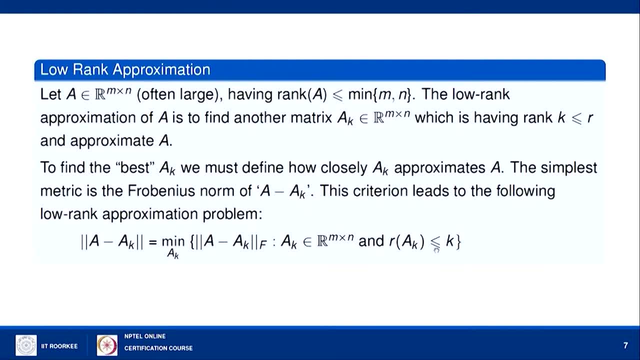 over all a k and rank of a k is less than equals to k. So this is an optimization problem. now We have to check whether it is a convex optimization problem or non-convex optimization problem, Because if it is convex optimization problem, 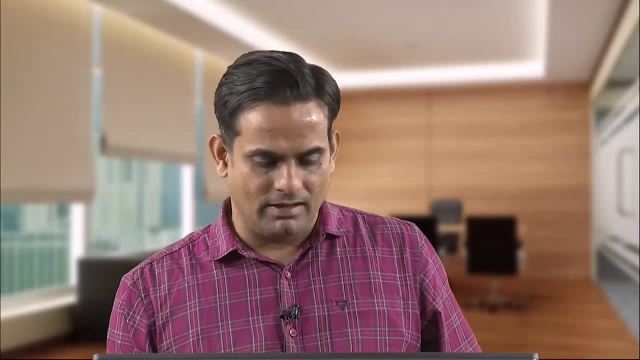 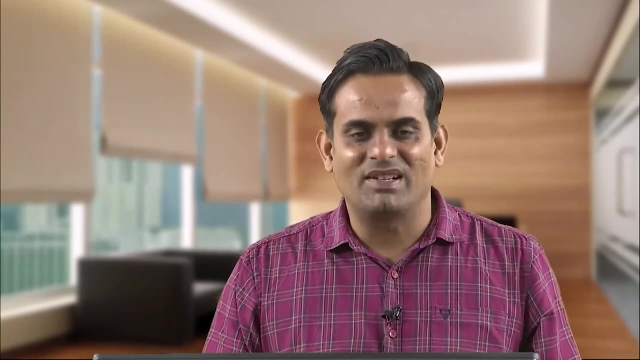 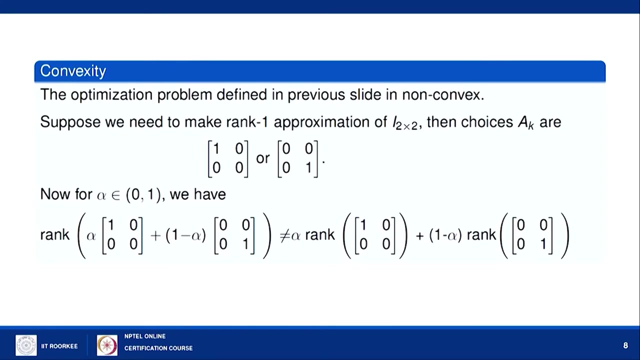 we can solve this problem quite easily. So now let us check. Unfortunately, this problem is not a convex optimization problem, So it is a non-convex. How you check with the help of this small example: Suppose we need to make rank 1 approximation of an identity. 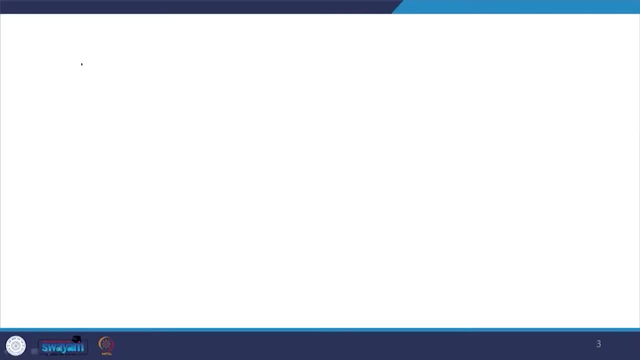 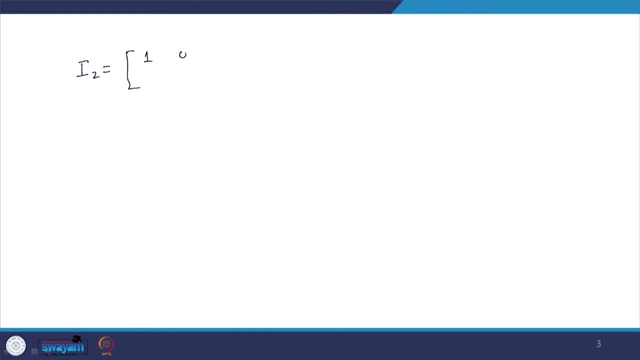 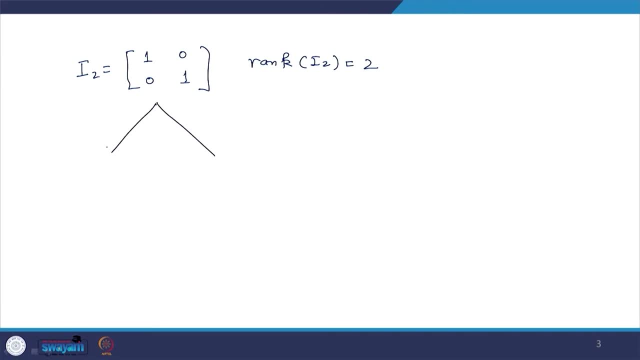 of this matrix. So you are having two choices: either you will go like this or you will go like this. So let us say I am saying this A and this I am saying B. So rank of A equals to 1 and 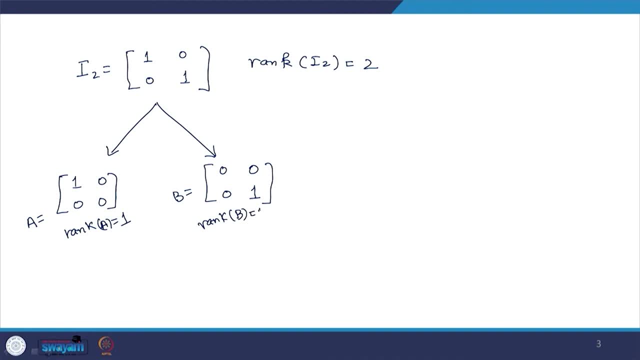 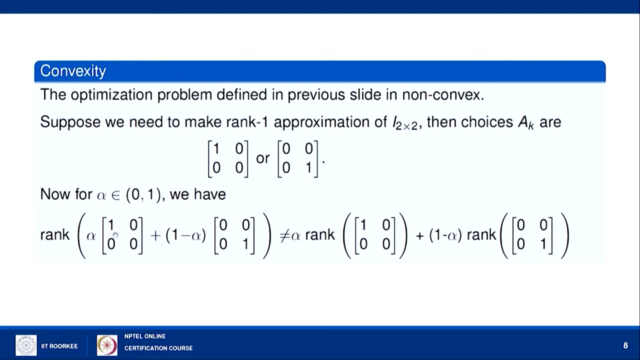 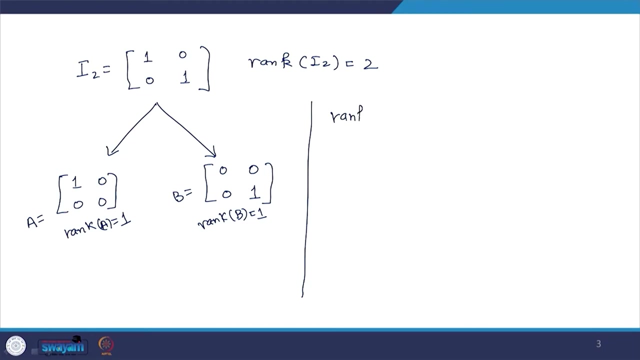 rank of B, again 1.. Now let us check the convexity of this. So now what I will do. I will find out, for some alpha belongs to 0, 1. Rank of alpha times A. So what I am having, Because here my function is rank, rank of. 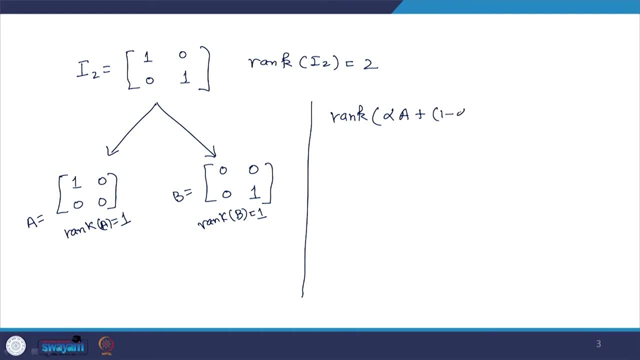 alpha times A plus 1 minus alpha times B, and for convexity it should be equals to alpha times rank of A plus 1 minus alpha times rank of B. So let us see whether this inequality holds or not. So first see alpha A plus 1 minus. 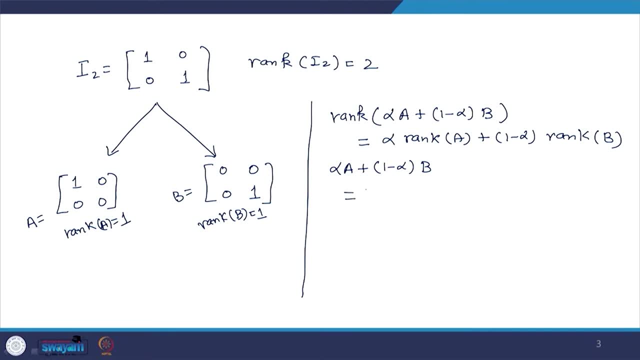 alpha times B. So alpha A will become alpha 0, 0, 0 plus 0, 0, 0, 1 minus alpha, and here alpha belongs to 0, 1.. So this will become alpha 0, 0, 1 minus alpha, and rank of this is 2 because it is having. 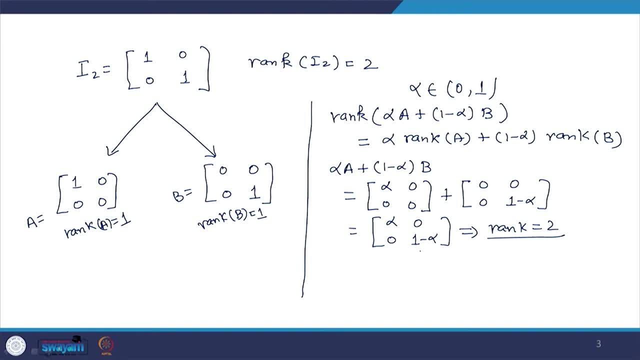 two non-zero rows and both are linearly independent. So this is the rank of this. one is 2.. So left hand side is 2.. Now what is right hand side? So alpha rank of A is 1.. So alpha. 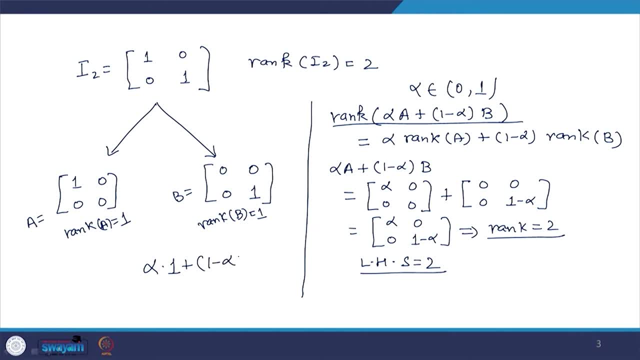 times 1 plus 1 minus alpha times rank of B. So I am calculating right hand side here. So again, rank of B equals to 1.. So it is alpha plus 1, minus alpha it is 1.. So RHS. 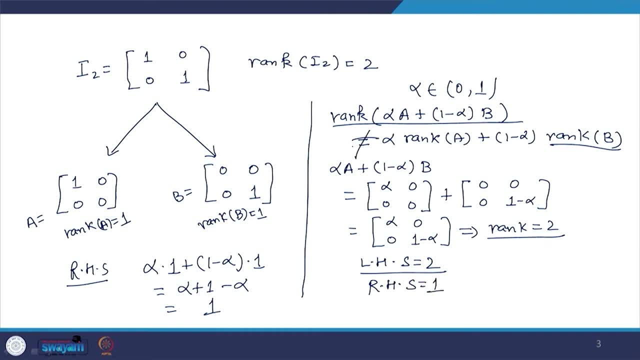 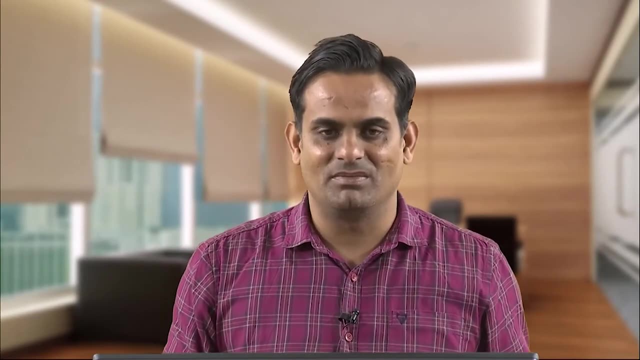 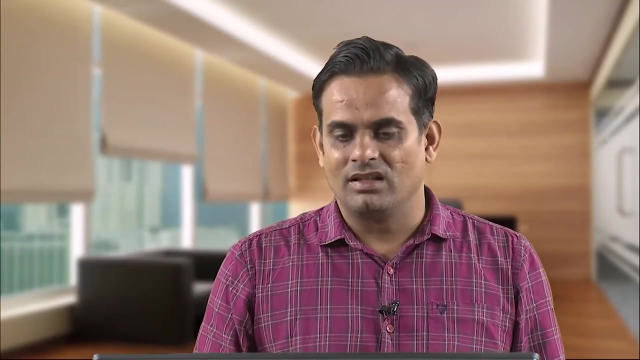 is 1.. So here this is not equal, and if this is not equal, hence it is a non-convex problem. Now it is very difficult to find out. the global minima of non-convex optimization problem. You will see in coming lectures when we will talk about gradient calculus. So what is? 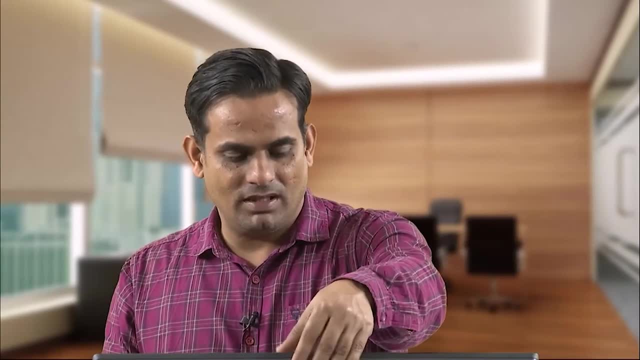 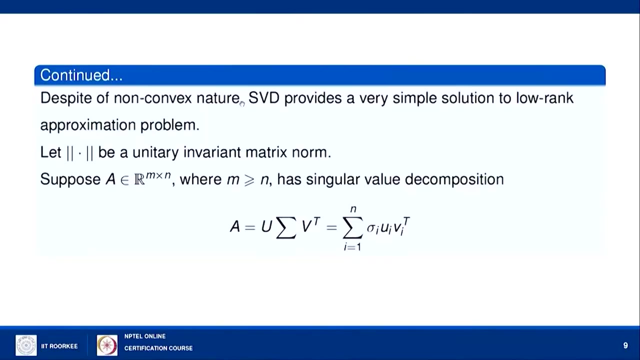 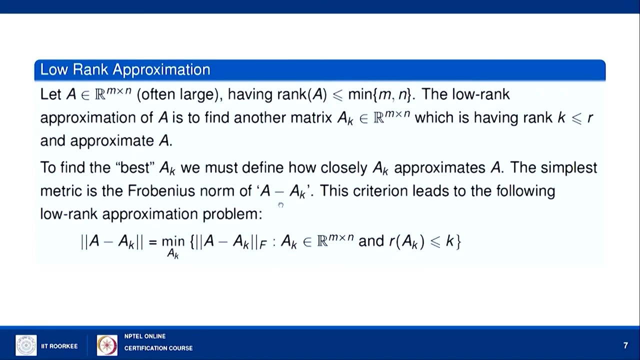 the solution. So solution come in form of singularity, So singular value decomposition. So, despite of non-convex nature, singular value decomposition provides a very simple solution to low rank approximation problem. that is the optimization problem which we have pause in this slide, this one. 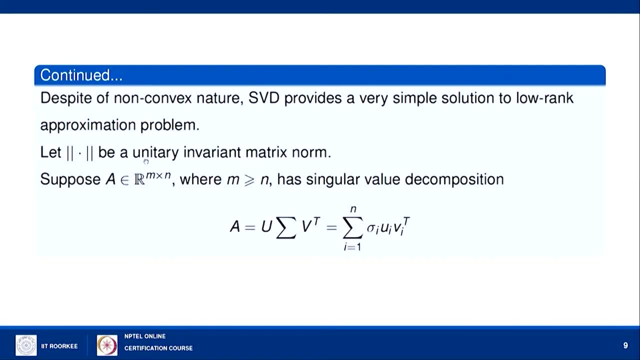 How let this particular thing be a unitary, invariant norm. And suppose A is a m by n matrix, where m is greater than n. We are taking this case, it is true for another case also, where m is less than equals to n. Hes singular value decomposition as A equals to: 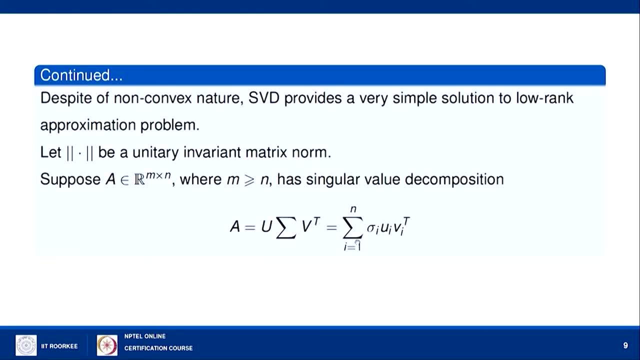 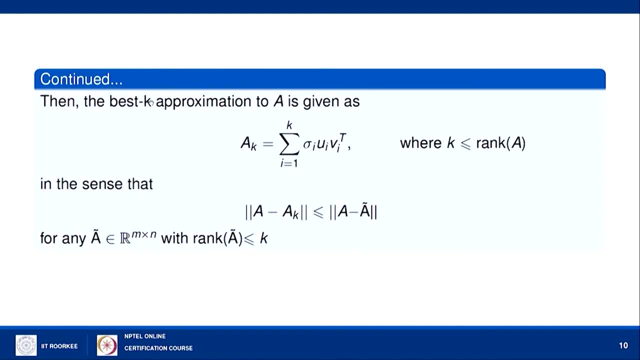 U. sigma V. transpose This. I can write also: I equals to 1 to n. sigma U i V i transpose. Now then, the best K approximation to A is given as A k equals to I equals to 1 to k. sigma i u i v i transpose: where k is less than equals to rank of a. So please see here. 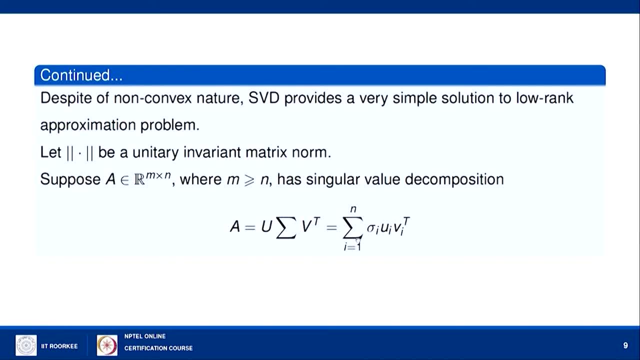 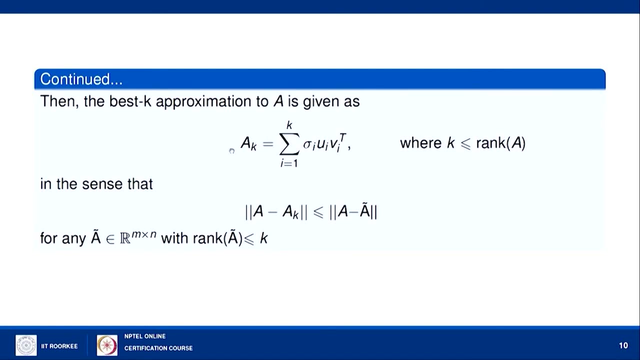 in this for the complete a, I am having this sum from 1 to n, So it will be having a decomposition over mean sum, over all singular values. However, this when I am talking about the approximation, I am having taking only k singular values. and what k singular values? the largest k singular 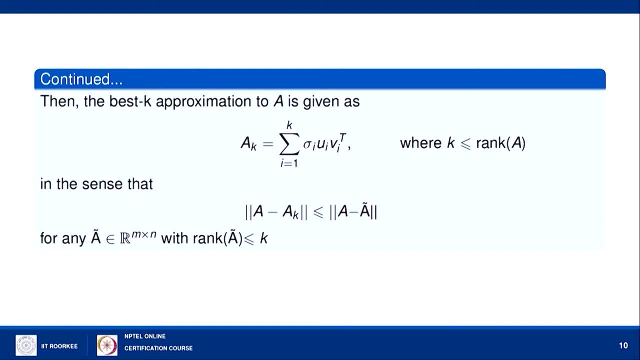 values After k singular values. I am making rest of the singular values as 0.. And in the sense that the norm of Frobenius, norm a minus a k or any invariant norm less than equals to a minus a tilde For any a tilde which is coming from the 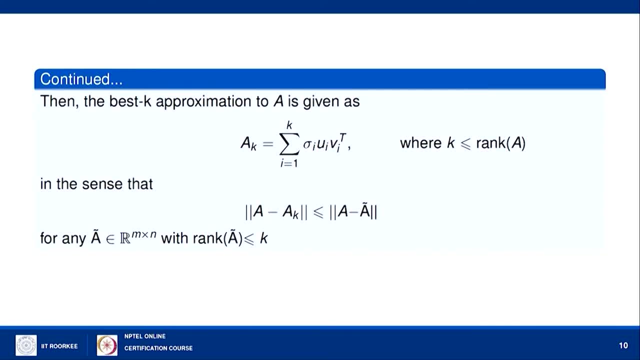 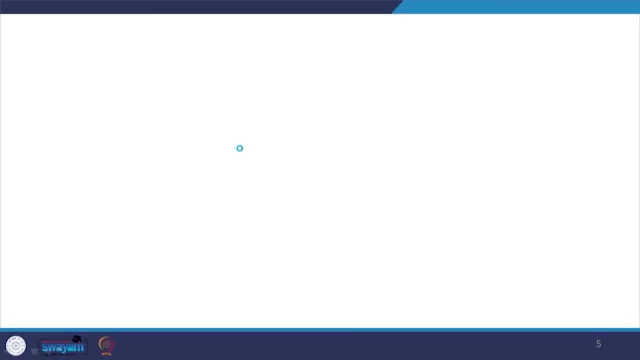 vector space of the matrices, a real vector space of the real matrices of size m by n, with rank tilde less than equals to k. So what I want to say, let us see by some simple examples. So let a be a phi by phi matrix with singular values, as, let us say, sigma 1. 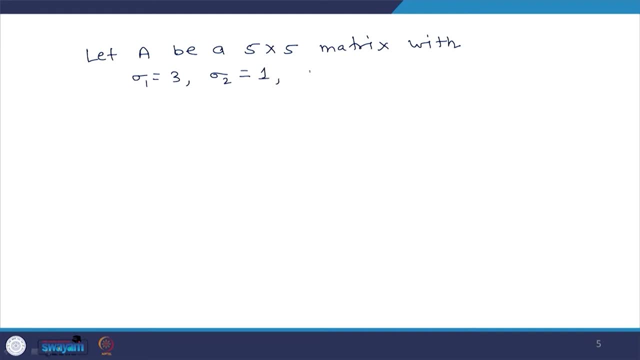 equals to k. So let a be a phi by phi matrix with singular values, as let us say: sigma 1 to 3, sigma 2 equals to 1, sigma 3 equals to 0.5, sigma 4 equals to 0.2 and sigma 5. 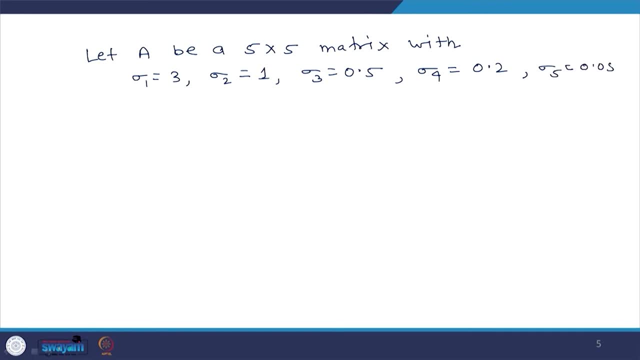 equals to, let us say, 0.05.. So what is rank of A Here? rank of A is 5, because all 5 singular values are non-zero. Now, if I want to find out A 3, which is a low rank approximation, 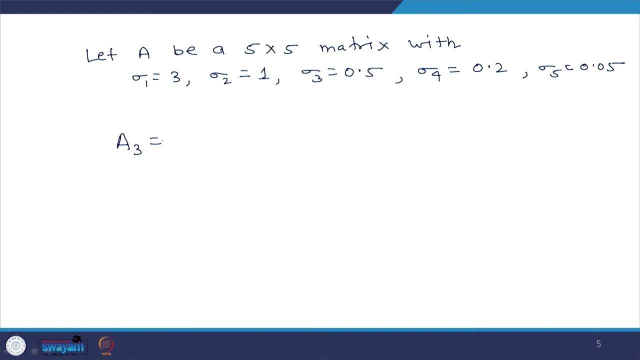 of A with rank 3, then what it will become. And one more thing: A equals to U, sigma V transpose. So now, what will be A 3? A 3 will be U. and then what sigma U will be. take Sigma 1, 0,. 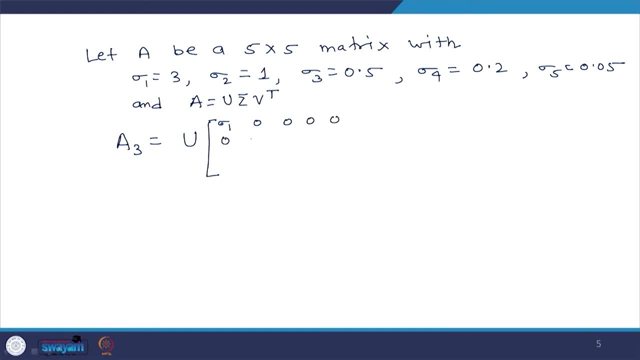 0, 0, 0, 0, sigma 2, 0, 0, 0, 0, 0, sigma 3, 0, 0 and then 2, 0 rows, Because if I want, 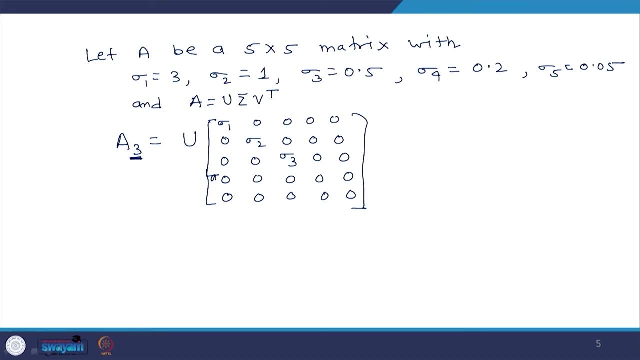 a matrix 3 rank approximation of A, then it will be having rank 3, and which is having only rank 3.. So if I want a matrix 3 rank approximation of A, then it will be having rank 3 and which will be 3 non-zero singular values into V. transpose Now what I want to say. if you 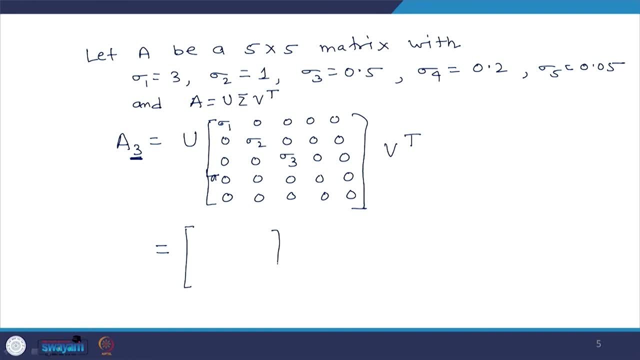 are having this matrix U, which is a. if A is 5 by 5 matrix, So this will be a 5 by 5 matrix, then I have written this sigma. So now ignore all these, because these all are 0.. So now, 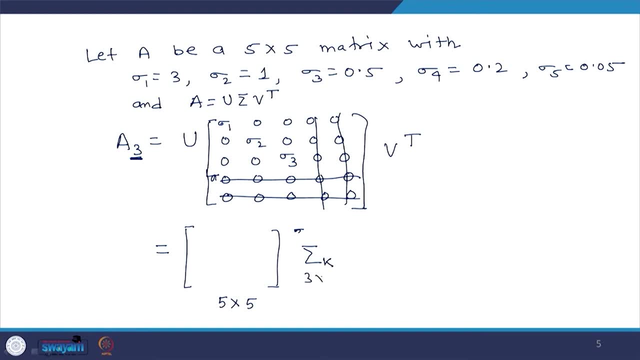 sigma k will become 3 by 3 matrix and then V transpose, which is again 5 by 5.. Now how you will define this product. So for defining this product, this matrix must be 5 by 3 and this will be 3 by 5.. So 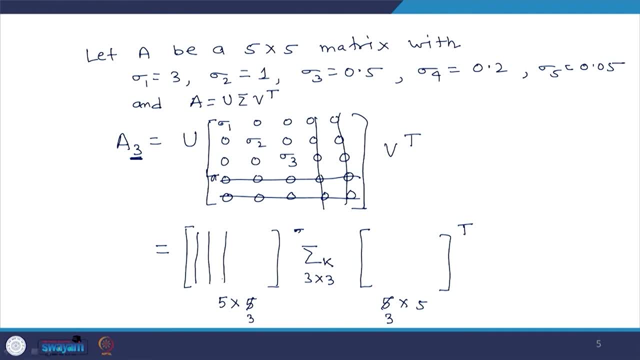 you will have first 3 columns of U and first 3 rows from here and then make this product. It will ultimately give you a 5 by 5 matrix and which will be having rank 3 as compared to rank 5.. So this will be the best approximation of the original matrix A and this will be the 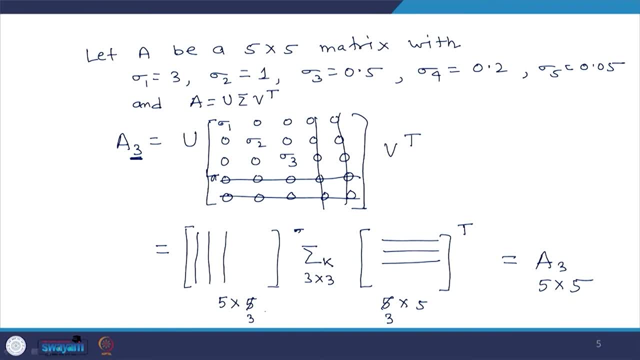 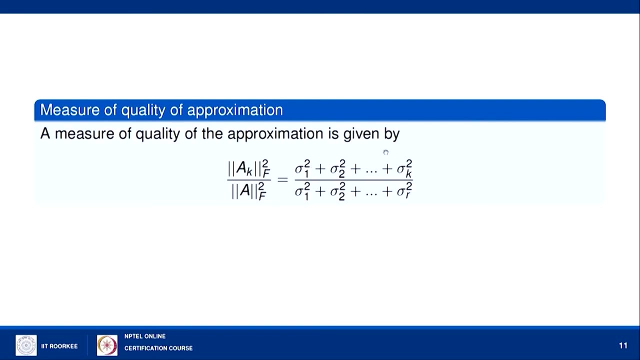 best approximation of A with rank 3.. Why I am saying it will be the best approximation? Let us see an example on it. And one more thing here. the measure of quality of the approximation is given by that. if you are going from rank R to rank k, where k is less than equals to R, then sum of the squares. 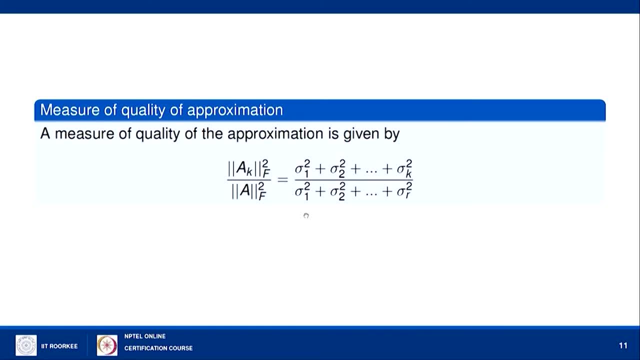 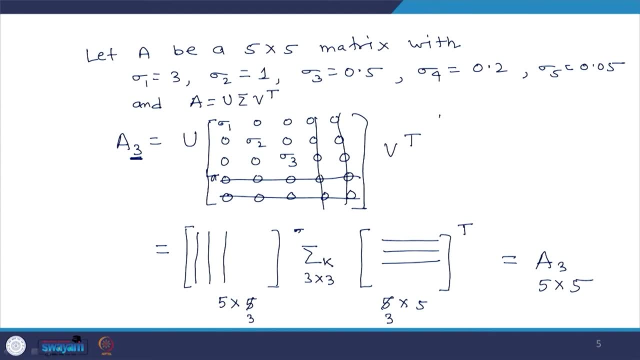 of the R singular values divided by sum of the squares of the R singular values. So for example, if you see here, here approximation will be 3 square plus 1 square plus 0.5 square. That is the first 3 upon sum of all. So 3 square plus 1 square plus 0.5 square plus. 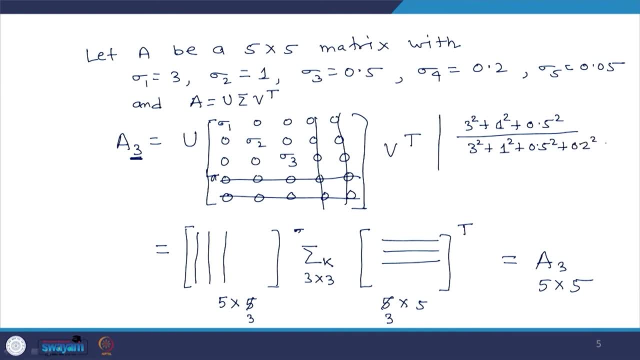 0.2 square plus 0.05 square And you see, if you ignore the singular values- those are quite close to 0 or very small- then quality of approximation will not be affect much. So in that way this is a measure or this is a metric for finding the quality of low-ranked. 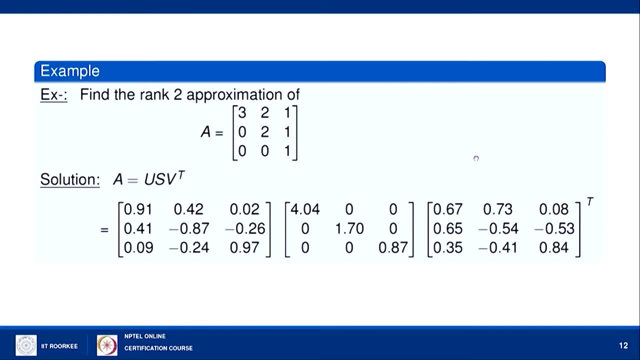 low-rank approximation. So find the rank to approximation of this matrix. So if you see it is a upper triangular matrix and the rank of this matrix is 3 because you are having 3 non-zero, linearly independent row. Now find out the singular value decomposition. 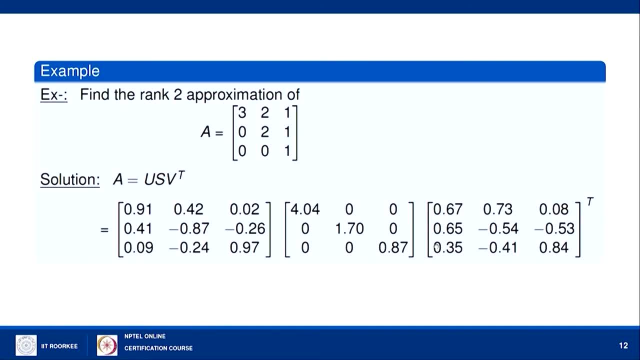 of this matrix. So singular value, decomposition of this matrix is given by: this is your matrix U, This is your matrix S and this is your matrix V. Now what you do? You have to find out 2, rank 2, approximation from rank 3, original 1, 2.. So what you do? You make this singular. 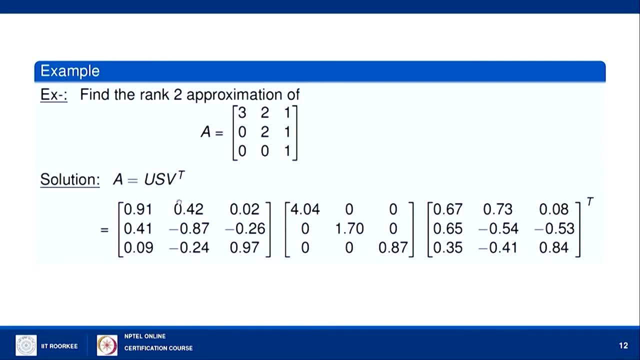 value as 0.. What you do? You take first 2 columns of this matrix. So instead of 3 by 3 matrix, you take this 3 by 2 matrix. Take this 2 by 2 sub matrix, So 3 by 2 multiplied with 2 by 2, and then that first 2 rows of this matrix, then 2 by 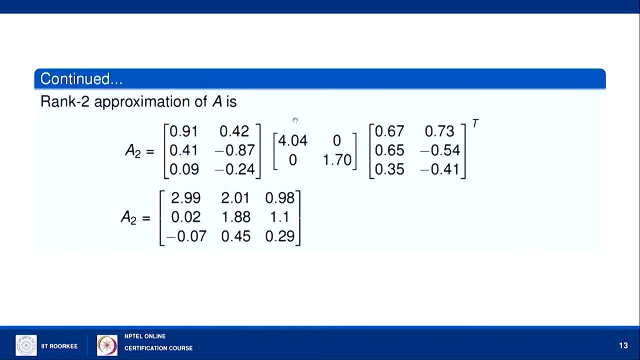 3, you will get this 3 by 3 matrix as I have taken here, and then this will be over. I why I am writing transpose? because once you take the transpose, this product will be defined. these are first 2 row only, So this will become the rank 2 approximation of the matrix. 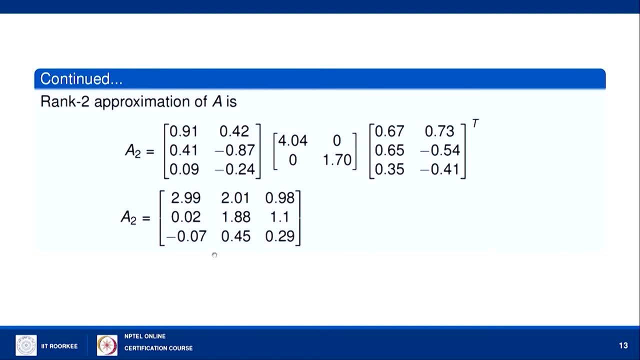 A. So rank of this matrix becomes 2.. So rank of the matrix A: 1, 2.. Now this matrix J is a very typical of this matrix because it is the complementary product, So in that of this matrix will be 2.. Now, if you compare this matrix with the earlier, the original, 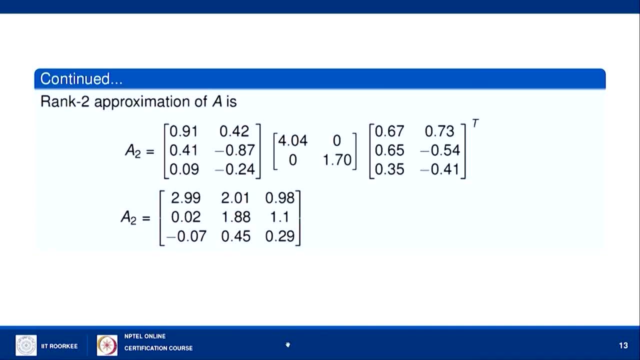 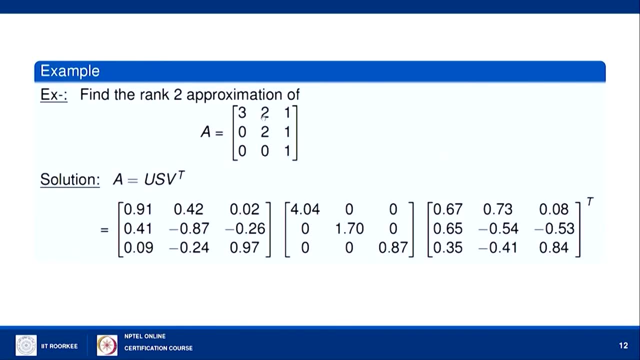 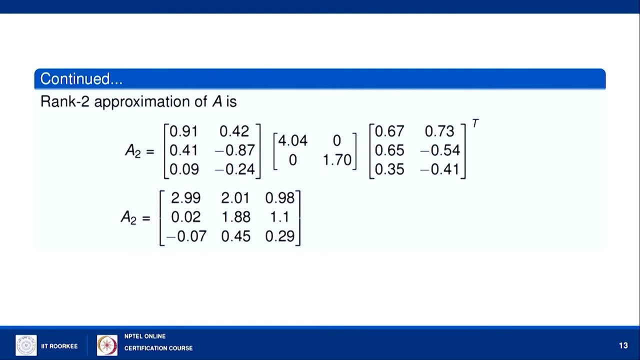 matrix. say, the first entry is 3, here it is 2.99.. So very close to 3. then here it is 2, it is 2.01.. So very close approximation. and the same time rank is reduced by 3 to. 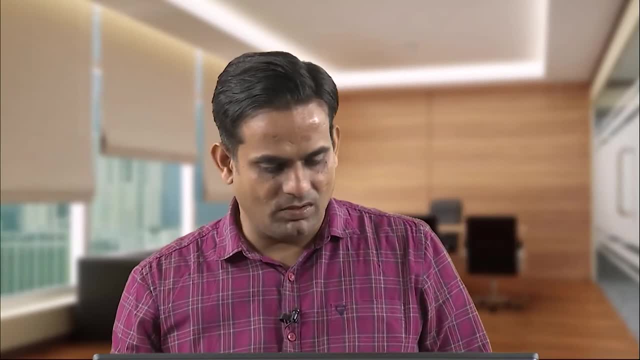 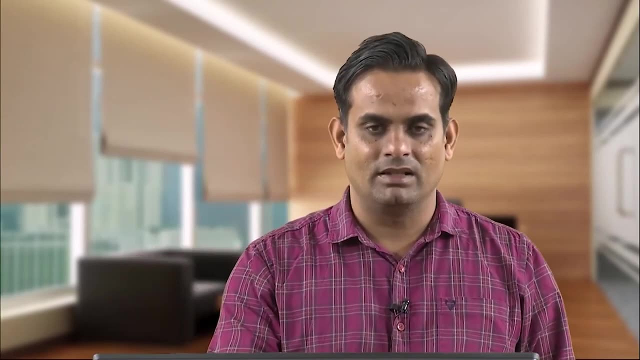 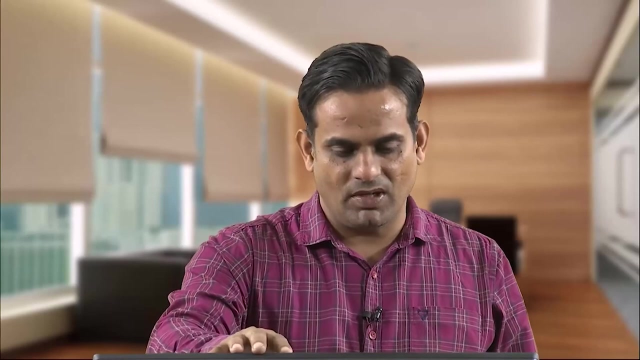 2. Okay, So this is one of the example of that for a smaller matrix, but generally we do this low rank approximation for larger matrix and where when we are dealing with learning of image use and all those. So let us see one example of digital images. 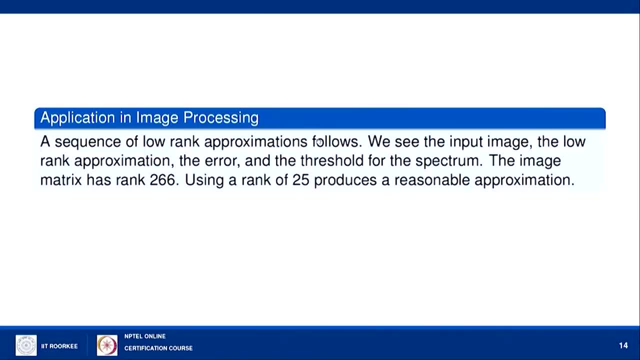 so we are having a sequence of low rank approximation. we have a, an input image, and we will find different, lower the error and the threshold for the spectrum. The image matrix has rank 266.. So the what is the rank of the image? 266, because image is a matrix only, So it is having 266 non-zero. 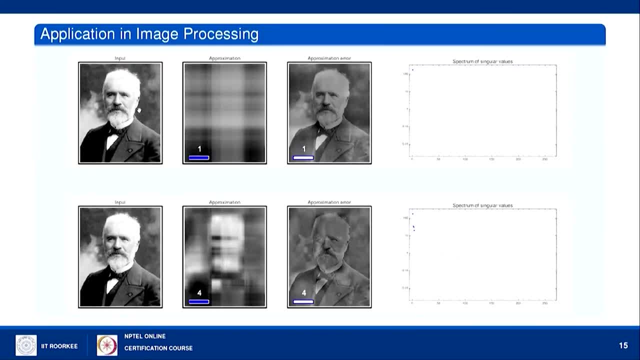 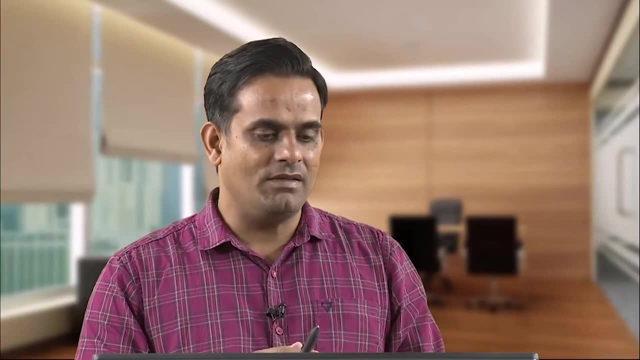 singular values. Now see, this is my original image, input image, which is having 266 non-zero singular values. So if I take only sigma 1, that is the largest singular value, then what I will be having. If it is a m by n image, I am having singular value decomposition m. 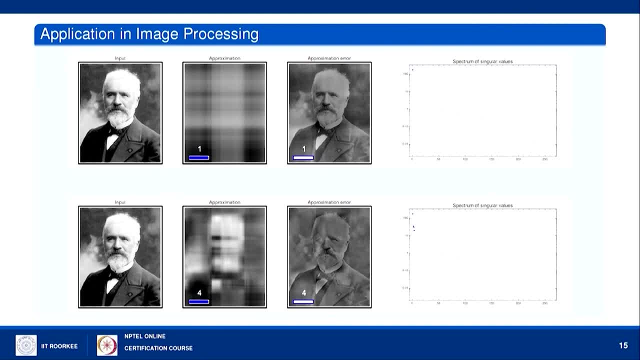 by m into m by n, into n by n. If I take only first column of U, first sigma 1, and then that is the U 1, sigma 1, V 1 transpose, Then I got this approximation and this is the error. Error means this minus this, or. 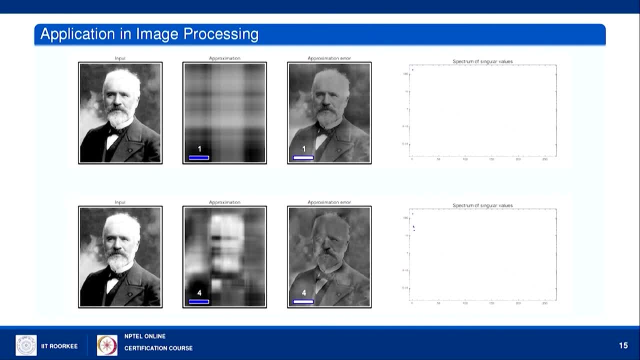 error means the image reconstructed from rest of the singular values, just ignoring the first one. So here it is not because you are having 266 rank and this is just rank 1 approximation. If you go to rank 4 approximation you can observe we are having some pattern which is 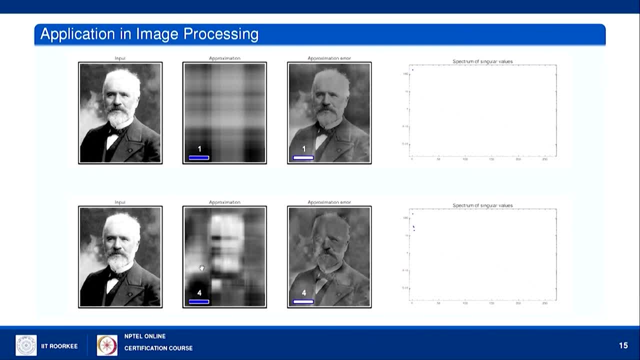 which are there in the input image. If we are taking more singular values, we are having better and better approximation. This is just spectrum. this is the first singular value and these are the first four singular values. Now this is the rank 10. approximation means. 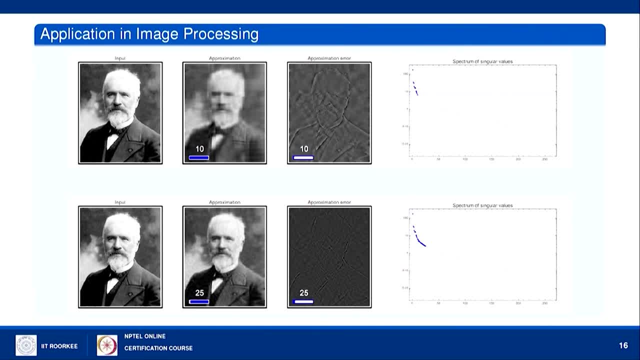 when you are taking the top 10 singular values and you are reconstructing or approximating your image. 266 rank image to 10 rank image. So this is the rank 10 approximation. So this is the rank image, rank image and this is the error. and these are the spectrum of. 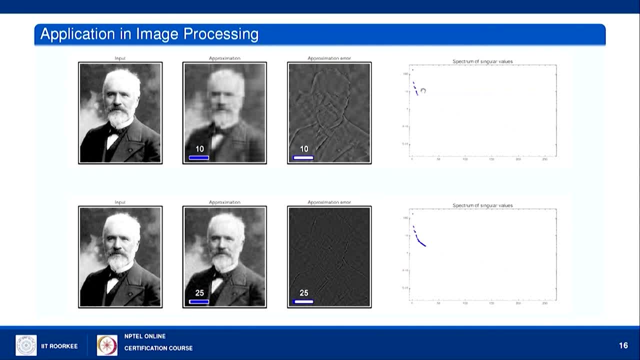 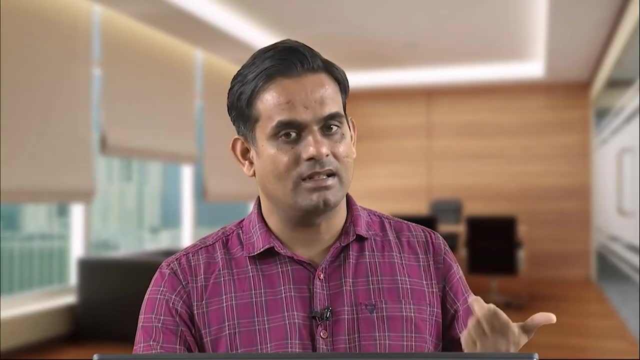 those 10 singular values. This is an example of if you are taking 25 top singular values in the approximation instead of 266.. Originally I was having 266, but here I am using only 25.. So you can see how.